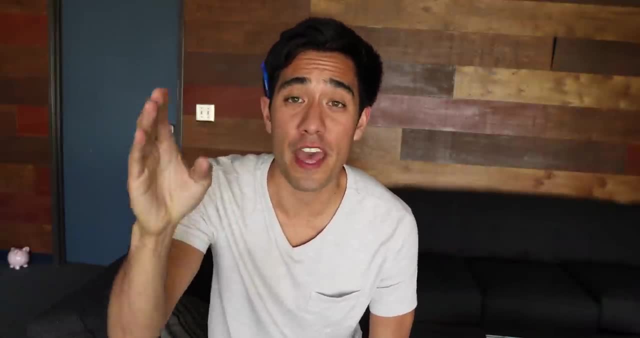 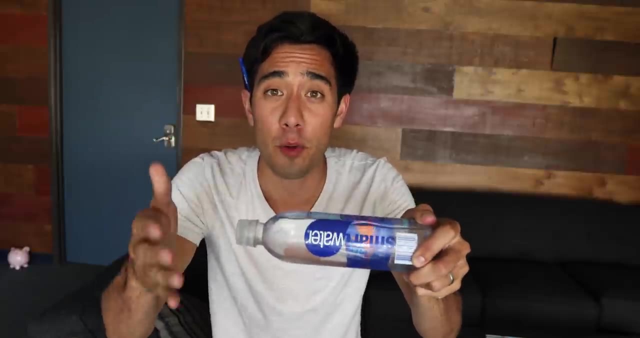 What's up everybody? Today I've got three magic tricks for you that you're going to be able to perform and show your friends using ordinary objects like a water bottle. Now, if you don't have friends, this will also help you get friends, like me, Anyway. keep. 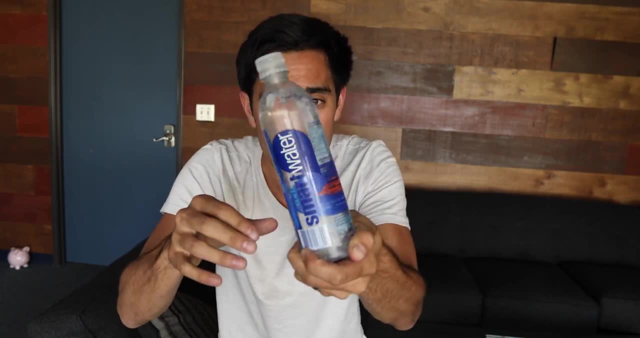 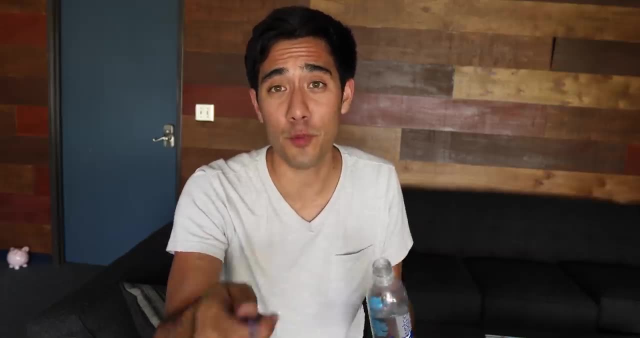 your eye on the bottle and keep your eye on this pen. Three, two, boom. And if you think this is some weird wizardry, I'm going to show you how to do it. Let's go to the park. I'll show you two more tricks. Cue the drone shots. 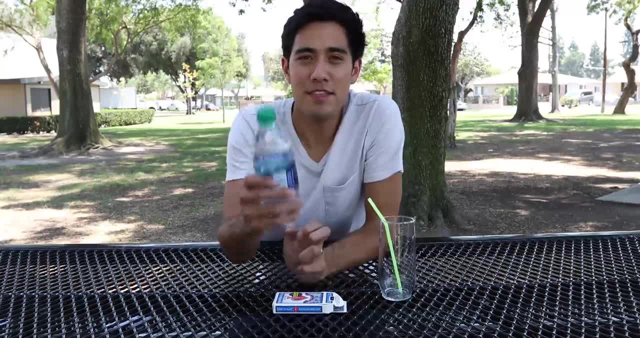 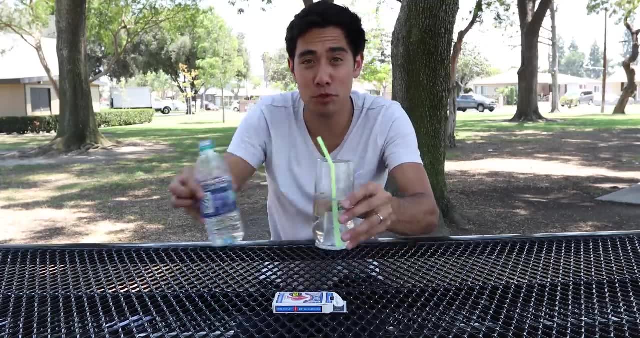 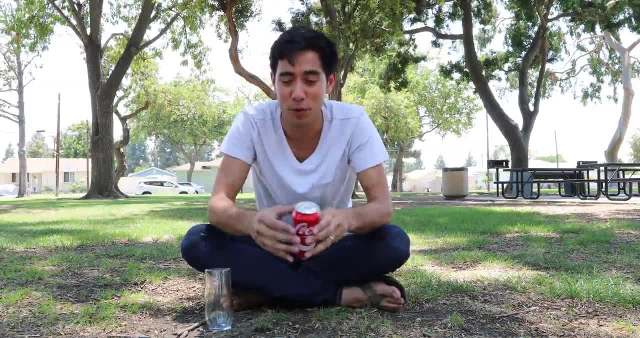 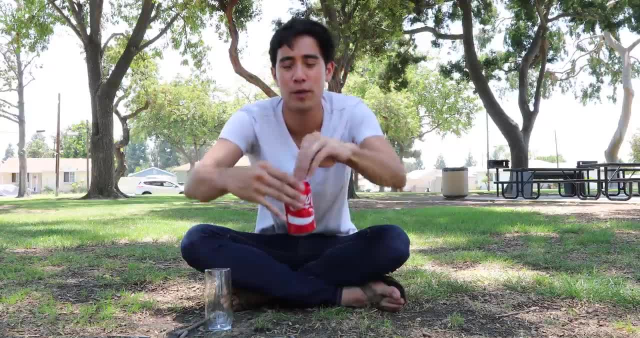 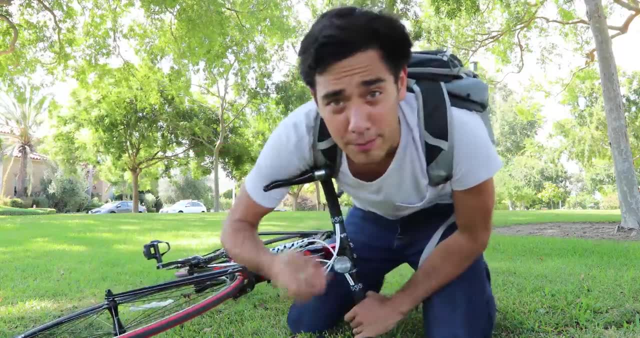 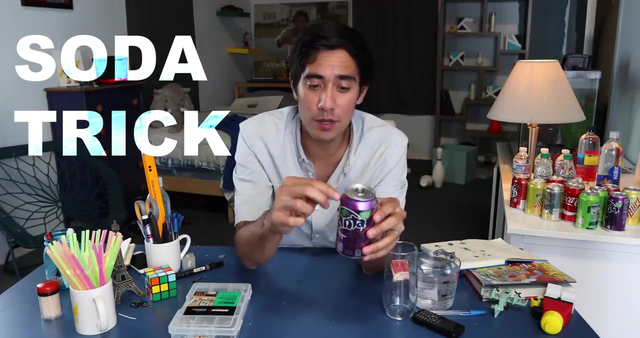 shake with the can and notice how it grows back to normal, right there in front of your eyes. so Cheers, we're gonna head back to my place and I'm gonna explain all of these tricks to you. you can do this trick with any carbonated soda or drink, but you got to make sure it has a can so you can puncture through. 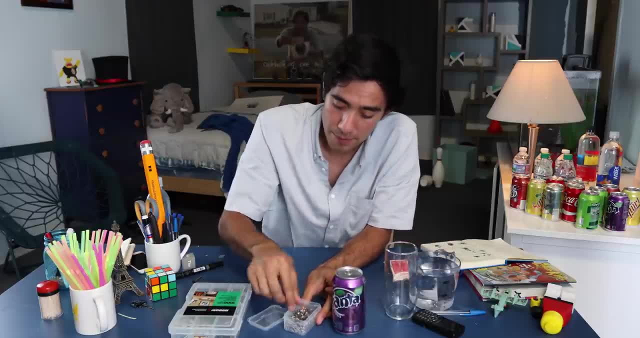 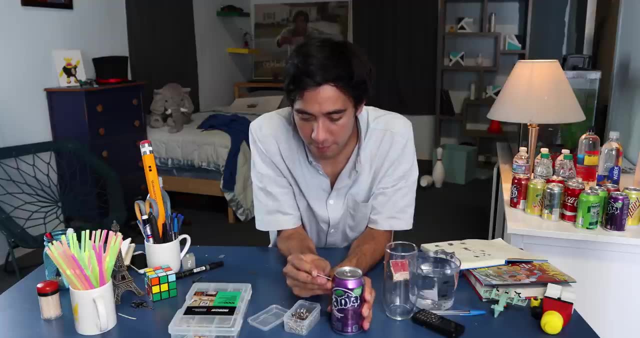 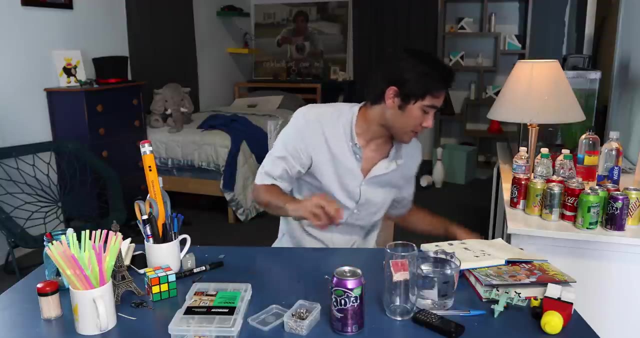 the aluminum. so what you're gonna do is take a bobby pin here, pull out the little needle. you could use a needle, but this is the best so you don't kill your finger. and before you do this, you might want to have a little protection, because this is gonna shoot out everywhere. so I actually usually do this. 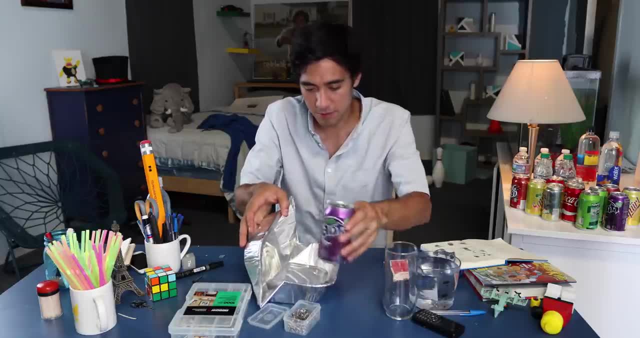 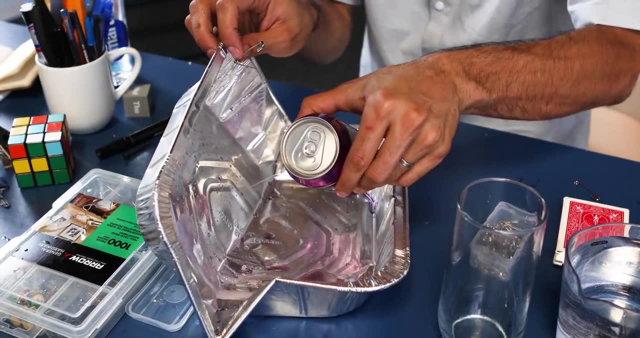 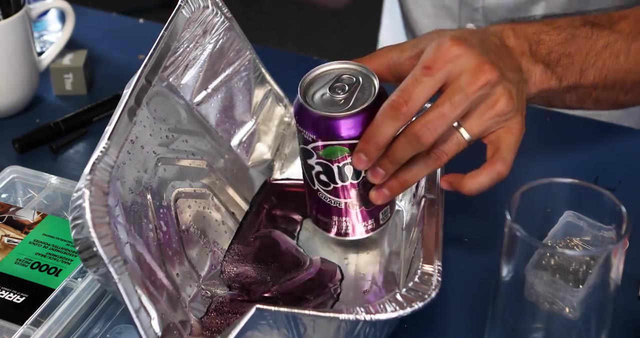 in a sink. but to show you, guys, I found this little thing in my garage and yep, and what you can do is continue to shake it. I like to get the cans about halfway empty for this trick to work, and once you pull it up like that, it'll stop. so there it is. you'll dry that off. 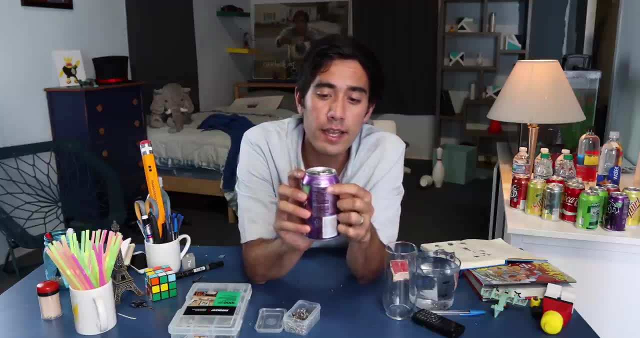 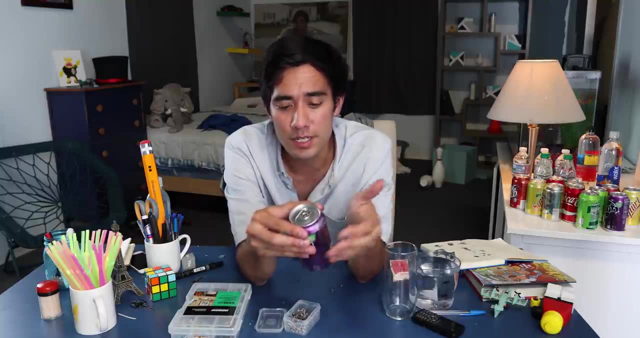 I like to usually put the hole in words on the back side here, but it really depends on the orientation of this. it's awkward if you have the hole here, because then you're kind of covering most the trick, which isn't fun because you can show this trick off like, just like this. so be here the second step of 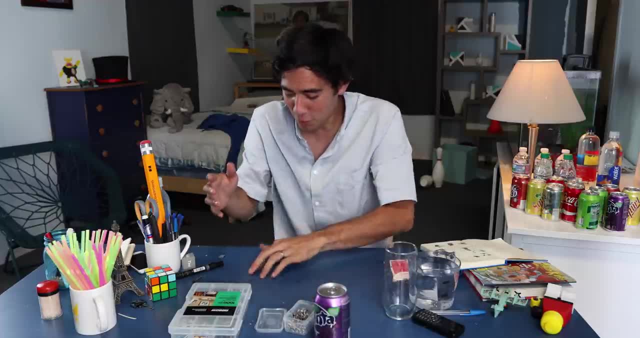 this trick is gonna be making this look like it's an empty can. this is a really cool illusion to me, because it's just, it's a real-life illusion. people aren't paying attention to this black piece of paper that you're gonna be using to make your can. 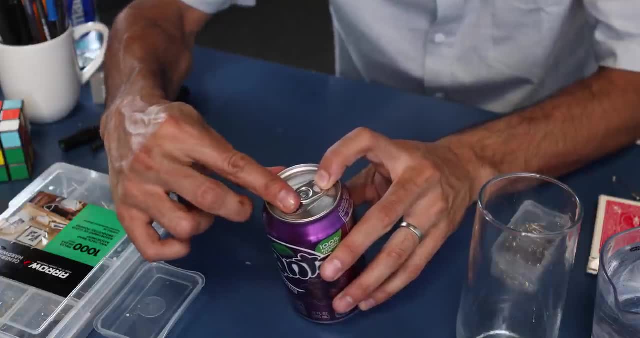 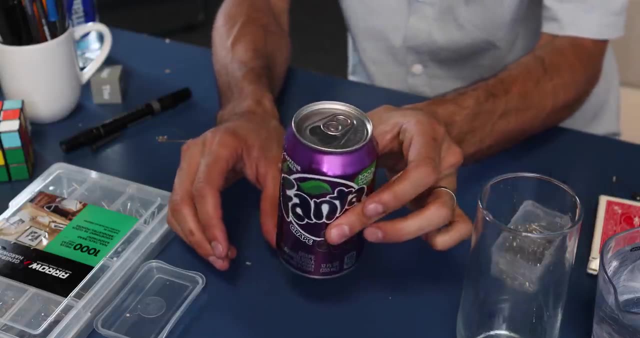 you can cut out in the same shape, slide it under the top there and in good lighting. so you got to be careful where you do this trick. it'll look like that is an empty can, which is just awesome. now you can just squeeze it if it's. 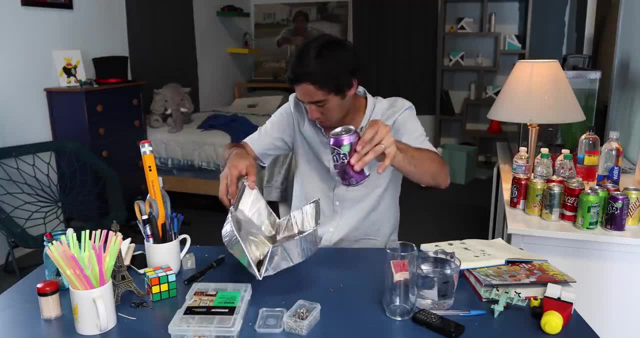 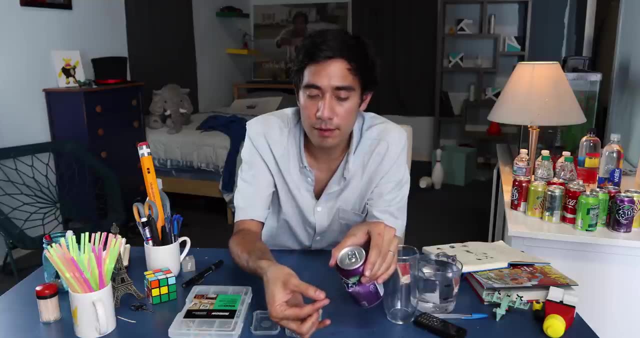 doing this. during the trick you're gonna want to empty that a little. darn it. I forgot that was in there. I just peed my pants, so you're gonna palm the top like that. that part's pretty easy, and then sometimes I'll crinkle it in my hand. 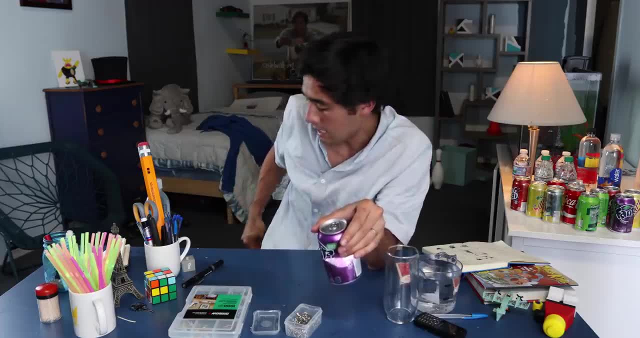 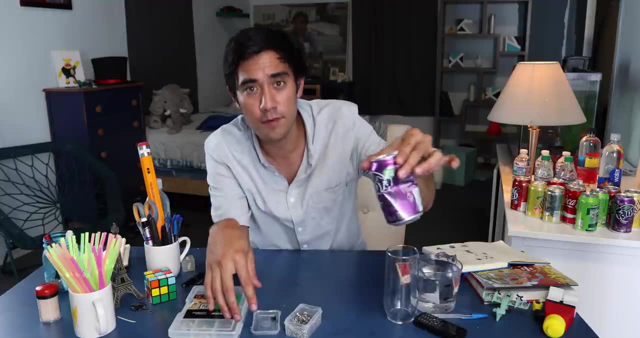 while they're not looking, let my hand naturally slide through the can and then swing down and put it in my pocket or crumple it up and kind of drop it and actually, while you're showing them this part that's falling to the floor and you're gonna step on that paper, the next part is gonna be shaking this can and 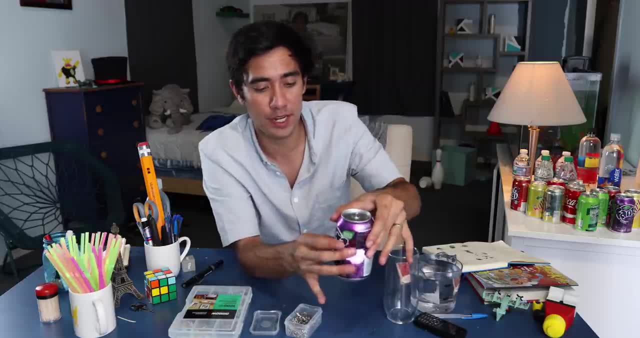 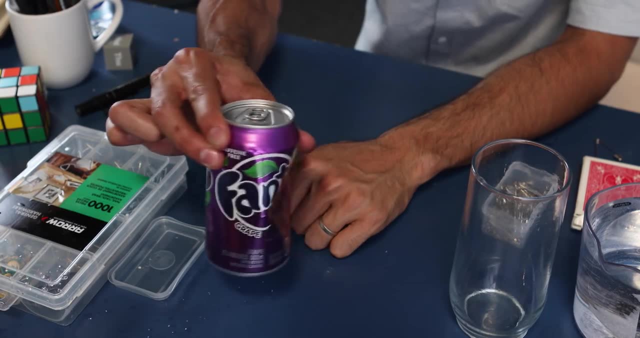 this is the cool part of the trick. it just it works, because of physics, with the carbonation, so you've got a bent here. so you're gonna shake this part of the trick and I like to rotate it like this, so it's not making sound with the. 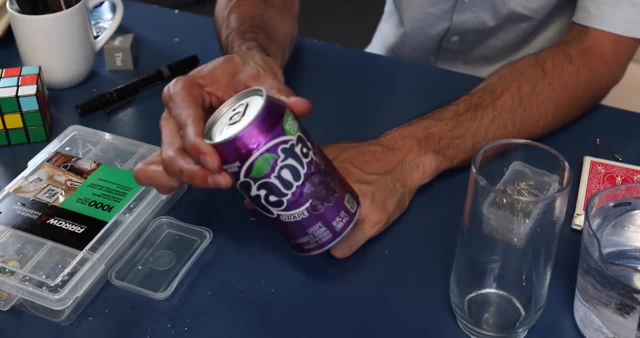 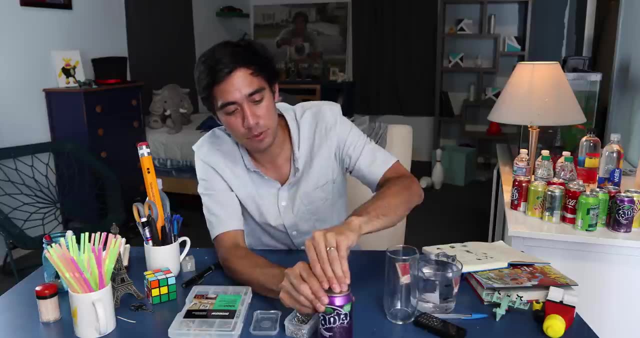 soda inside and you're gonna see it that's now inflated. you get the idea. and if you were let go of that hole? so you want to quickly open this up, and part of the trick is quickly pouring it too, so they can taste it, they can see. 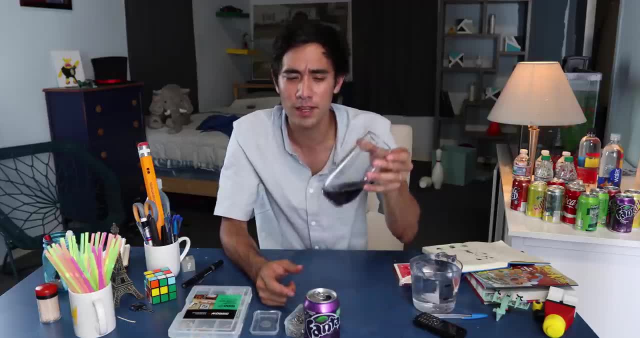 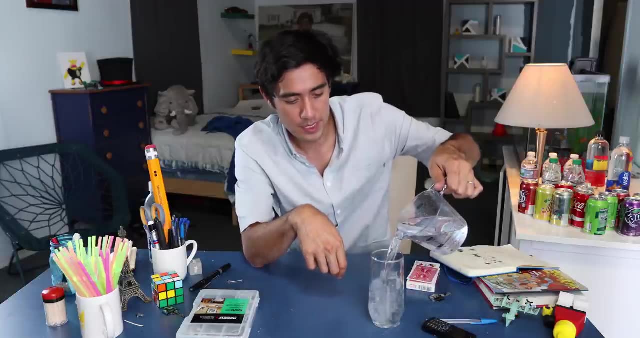 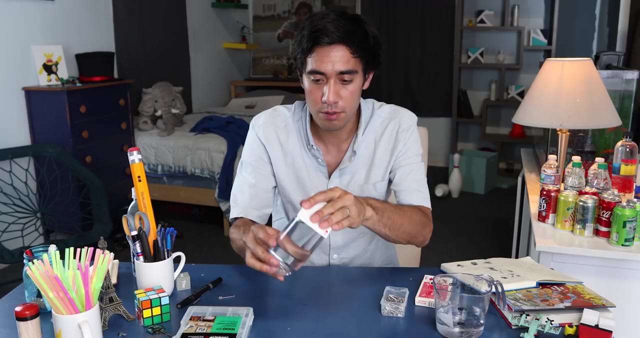 liquid coming out and that really sells that. what the heck they were soda in the whole time. I love this trick because it's fun. it's physics, it's real. there's a lot of practice that's involved. I'm gonna explain the concept of what can happen. so you have a car and you can use this in your performance to to show your 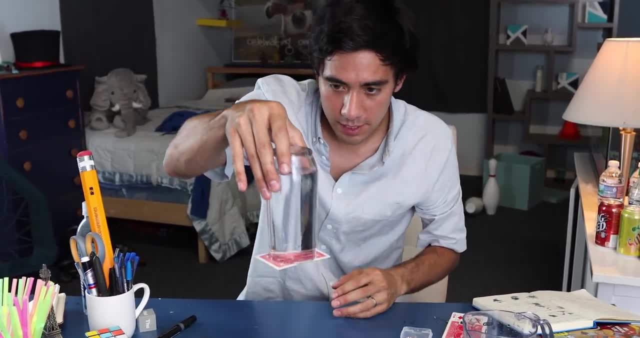 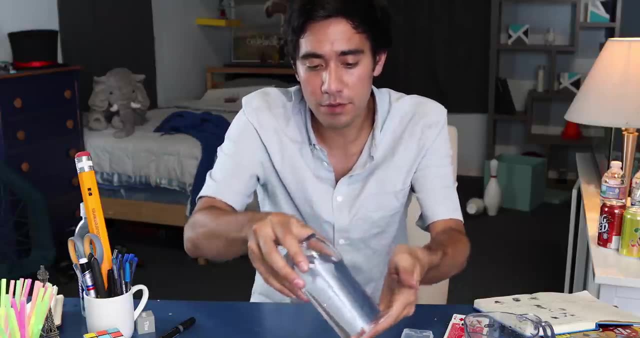 friends, but you show surface area tension. I don't know what the physical term for this is called, but the pressure of the air is holding the card up and if I took the card away there it's gonna fail. all the waters obviously gonna fall out. to perform this trick you're gonna want. 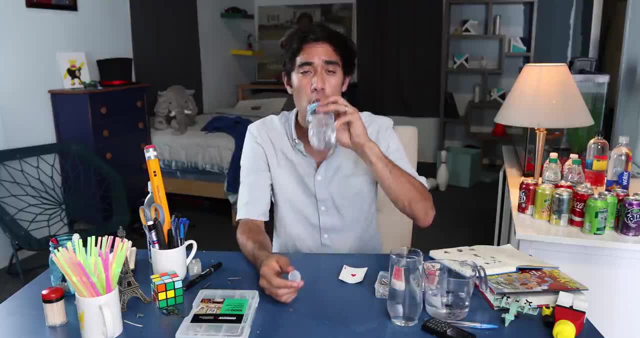 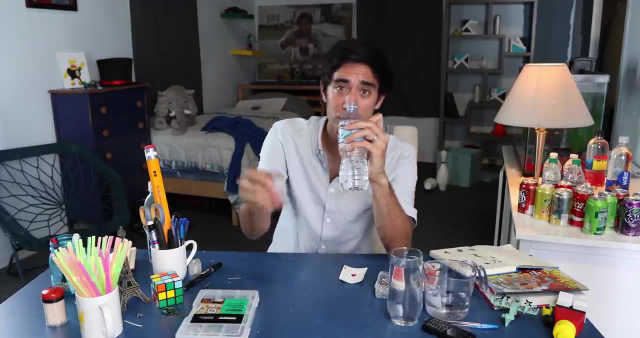 to grab a bottle of water and what I first do is take a swig and I'm proving that's a real water bottle. but I'm also showing this air pocket here, which is gonna help for this next part of the trick, because I'm gonna put a card in. 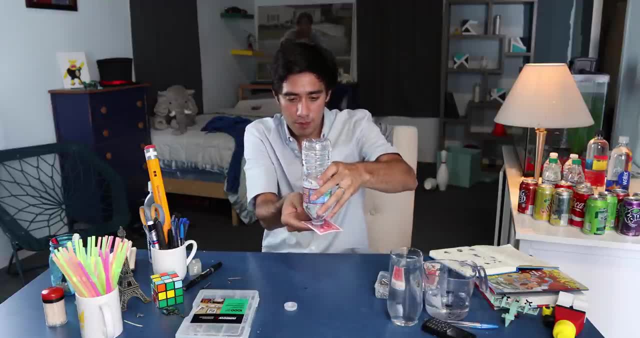 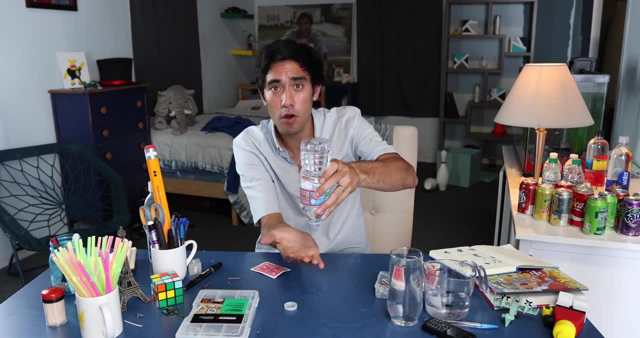 You can do it with your hand too. if you get a lot better, You pull it away, just right. you're going to have the effect nice, You can also do that again with your palm, and I'll show you that in a second. but what? 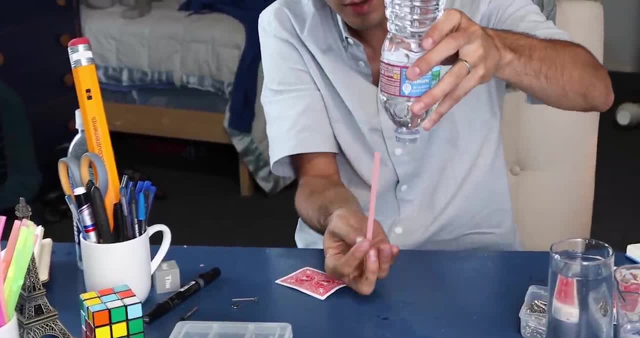 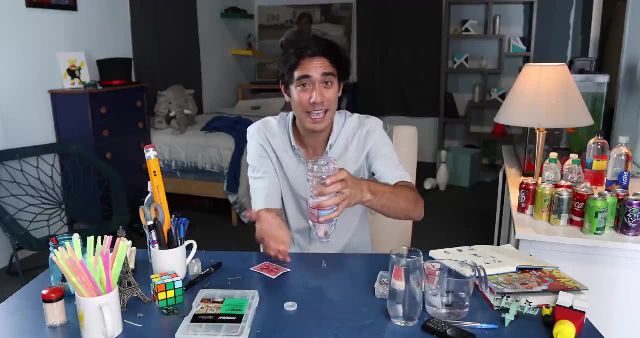 you're also going to be able to do here. this is the part that takes a lot of practice and you get the straw in there And what you can do is, if you can quickly turn it over- I can't. it usually messes up. 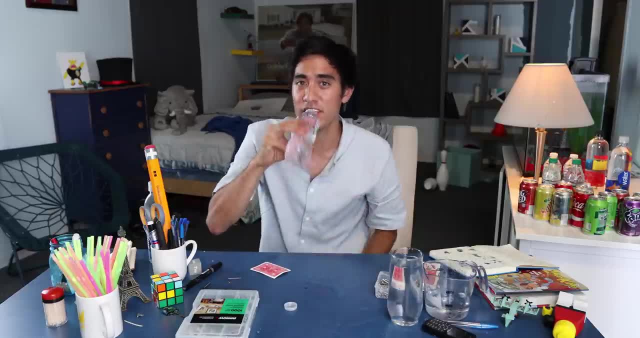 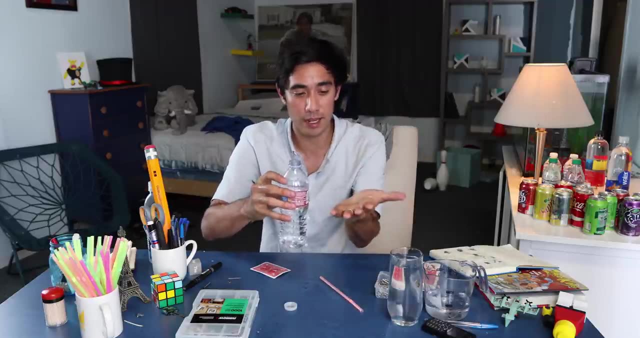 so I kind of pop it over and then you can drink out of it again and take the straw out. You can do whatever you want. So what you're going to do, if you want to do it with your hand, a lot of people like 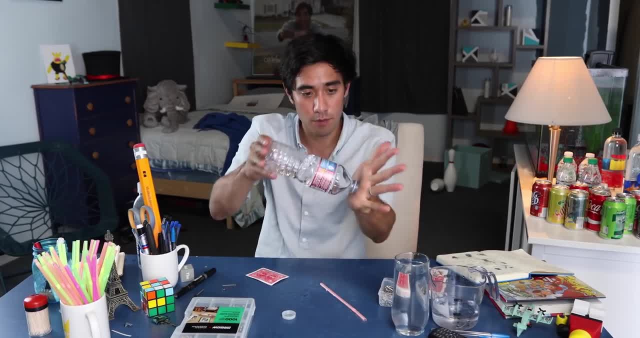 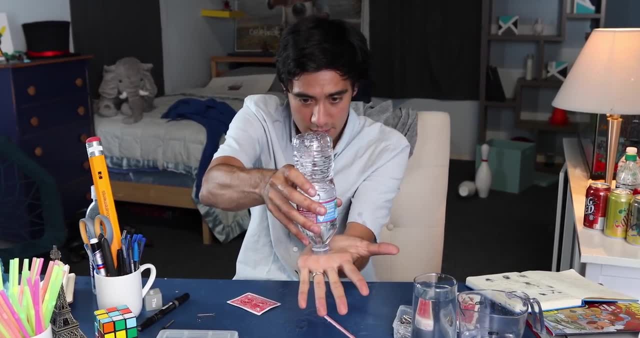 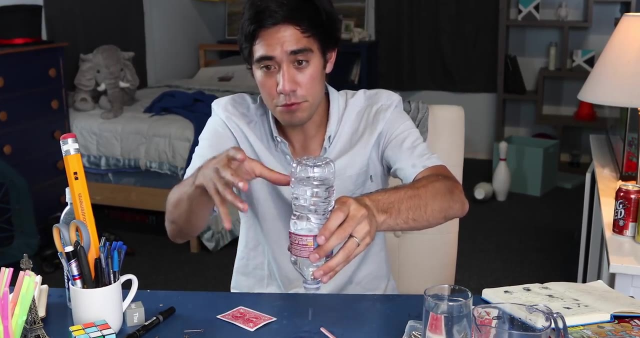 to put their hand top in the beginning and turn it over. And this is the part that's hard. you've got to be really stretched out and then you're going to slide it off like that. And when you get there, When you get it, if you squeeze this water bottle at all, all of this is coming down. 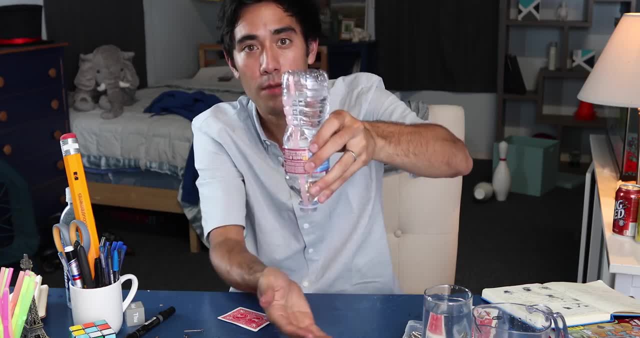 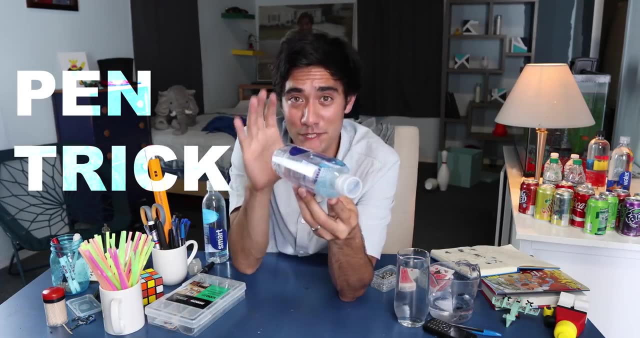 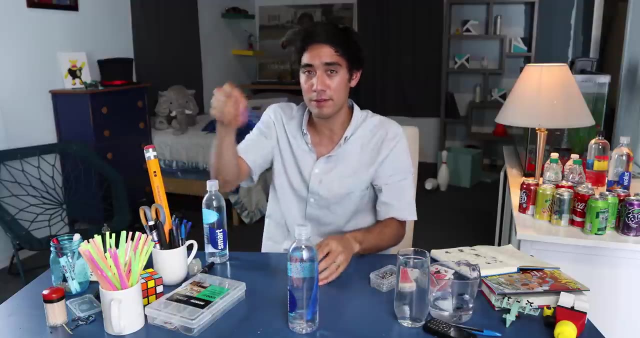 So you've got to be really still with it, and then you just pop that up like that. Now my desk is sticky and wet. I love this pen trick because what's going on is the pen is in there the entire time, So you're going to need a duplicate pen. 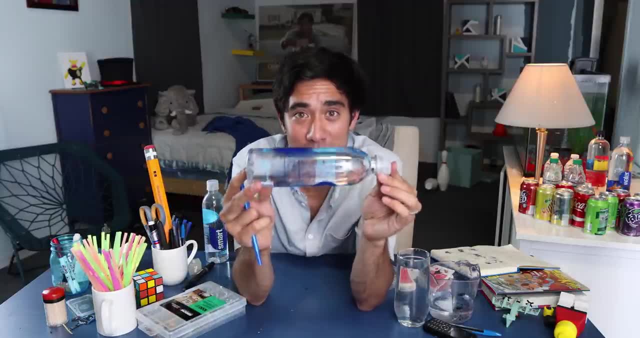 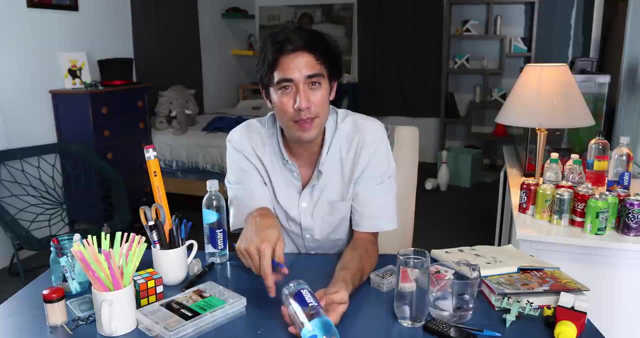 Go ahead and grab this here, And it's simple light refraction guys. This is how it disappears. You can't see it. So you've got to make sure you're performing this at the right angle, And if you're going to your friends too low, they might be able to see the pen maybe sideways. 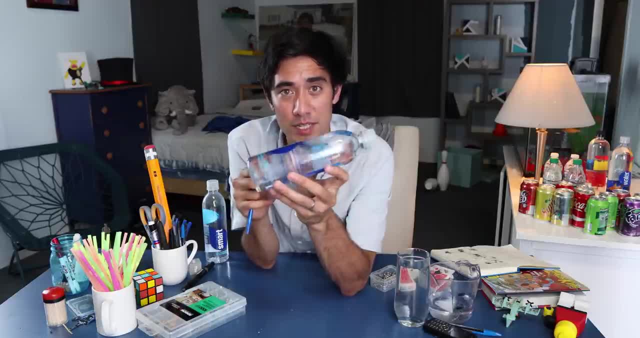 They can definitely see it. But right here is a sweet spot. I kind of point it towards camera a little bit. or you can go straight on, You can move it to prove: Hey, there's no pen here if you do a slow one. 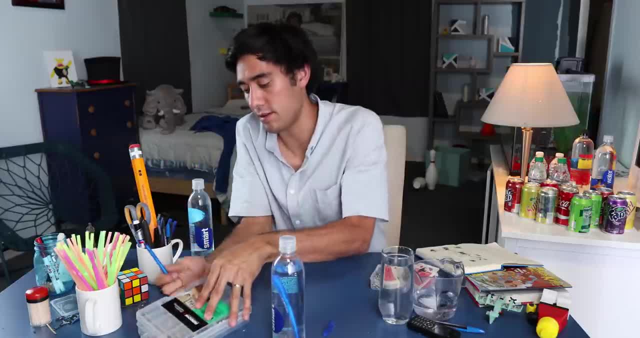 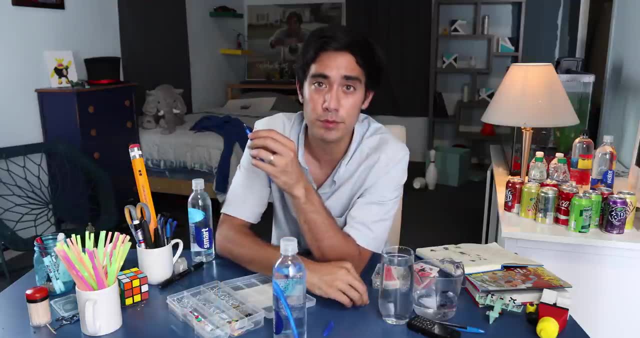 But what you're going to do is open up a pen and you're going to fill the inside of the pen. If you pop it off, however, these pens break open. fill it with tiny nails or weights. Some people do little ball bearings. 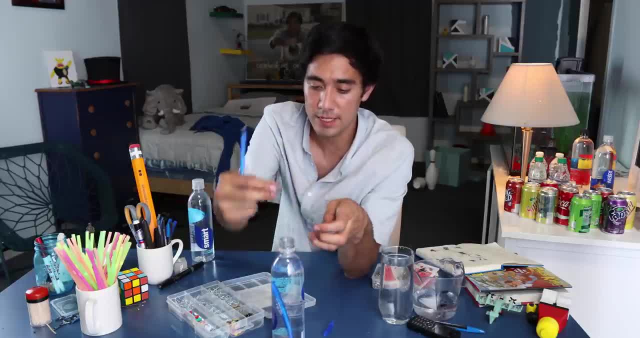 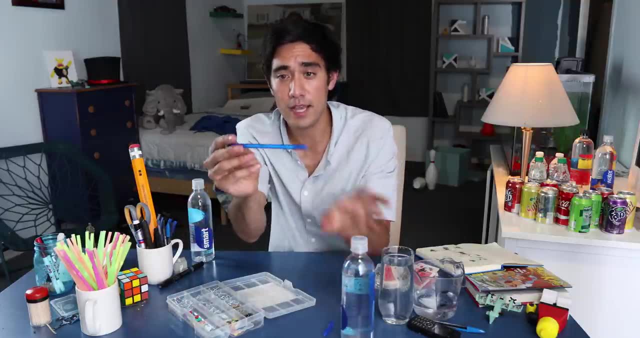 You just got to wait it down. So when you put the pen in here It's going to sink. Otherwise, a regular pen, this one's going to float like that. So get it weighted down, Do the trick like this. The back of your hand. you're just going like this for the performance. 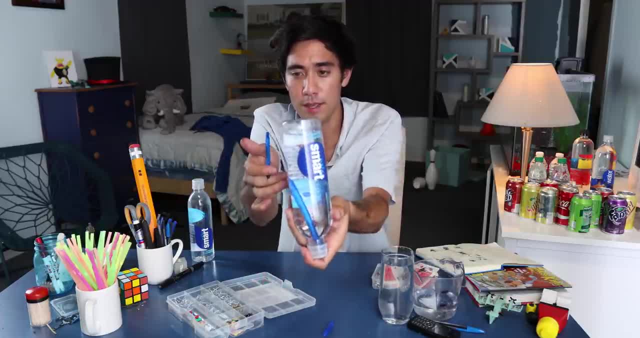 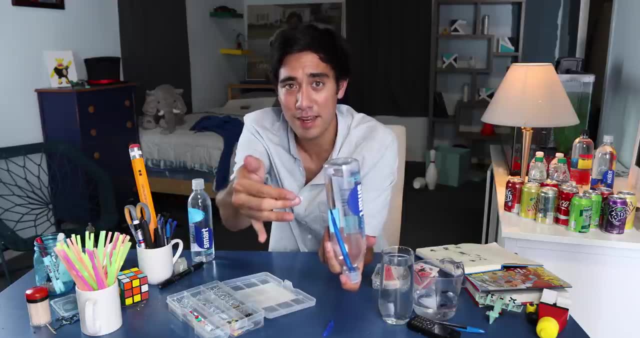 You're saying boom and boom And this is is just coming in here like and hiding your palming the pen. They're not paying attention to it because they're looking here and you're kind of hiding it, angling it behind here for a second. 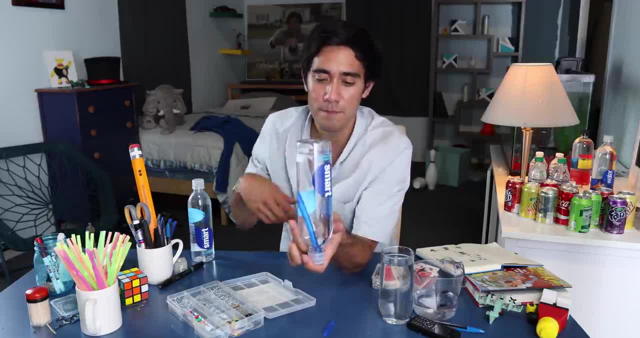 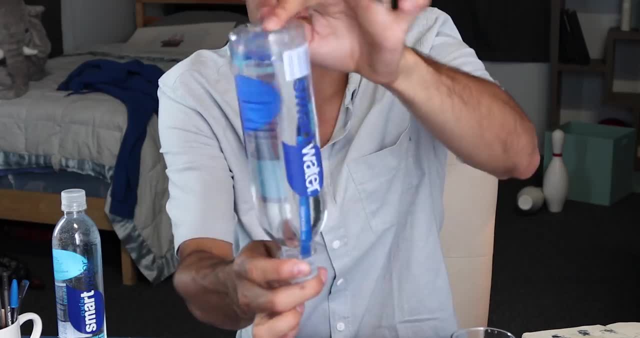 Then let your hand fall down, drop the pen in a pocket or give it to a buddy. that's in on the trick. There's all kinds of ways that you can get rid of the pen. but I'm just going to do this and like that and you show this pen and I can also show my sleeves or my arms.